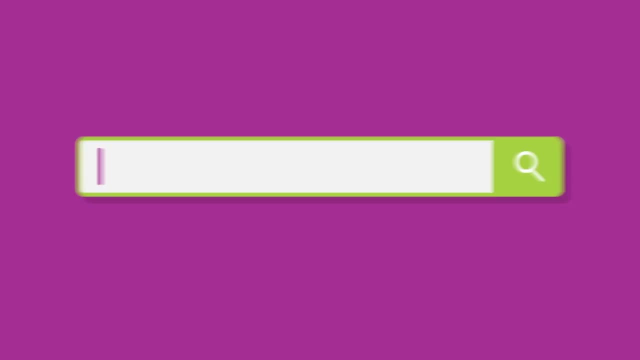 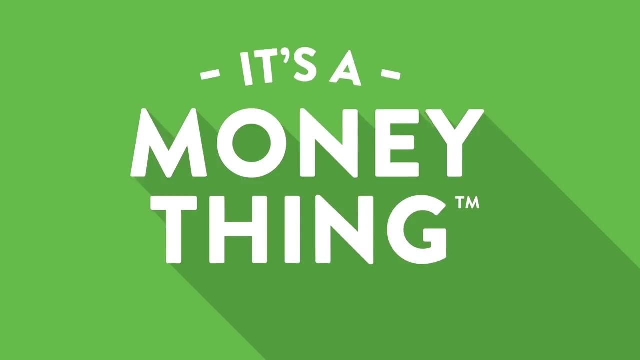 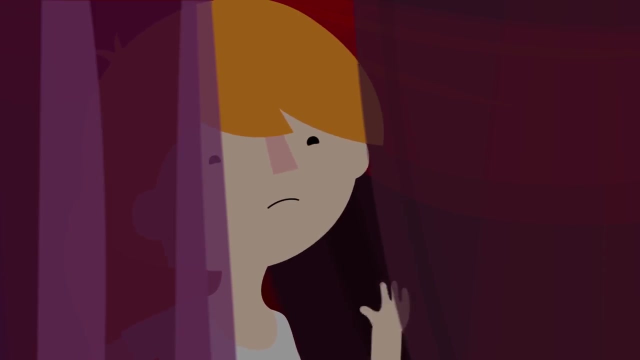 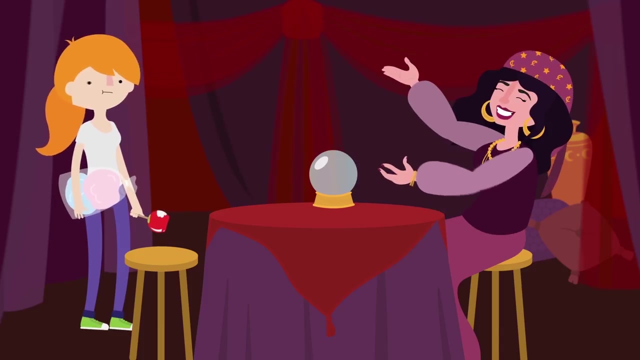 Portion teller. Ah sweet, I can't pass up a good deal. Come in, come in. Cross my palm with silver to unlock the secrets of eternal prosperity. Um, It's 20 bucks. kid What I mean, of course. I thought this was supposed to be a cheaper place. 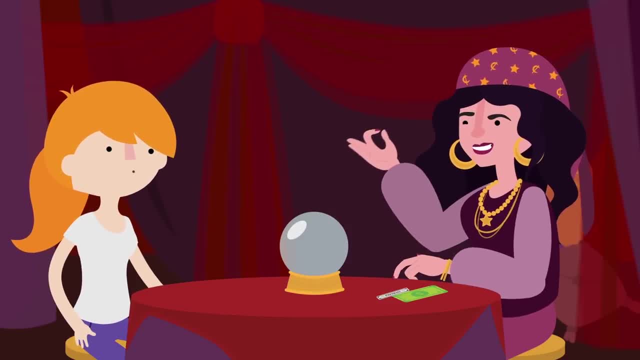 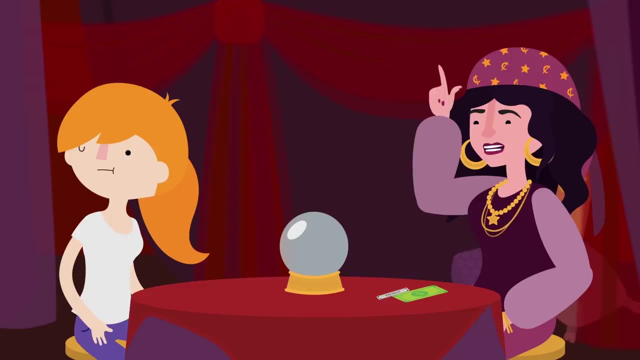 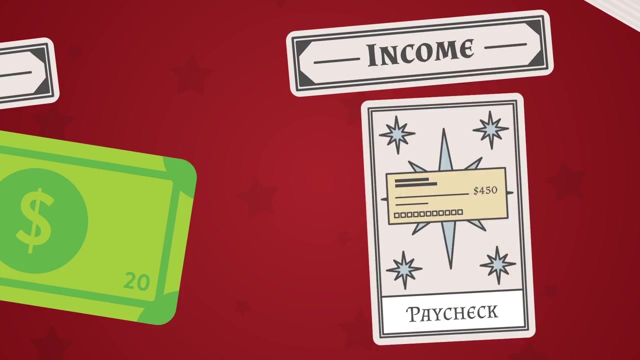 I sense, I sense your name is Jen, Jen Wow, And you appear to be a plumber. Nope, But there's more than meets the eye, For you have some sort of part-time job, Yes, Great. So you have a regular paycheck coming in? Draw a card, Jen. Choose wisely. 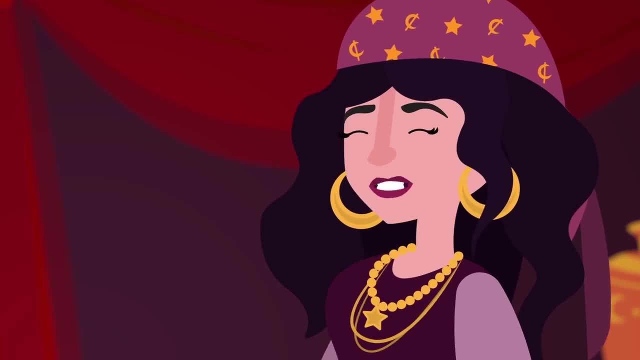 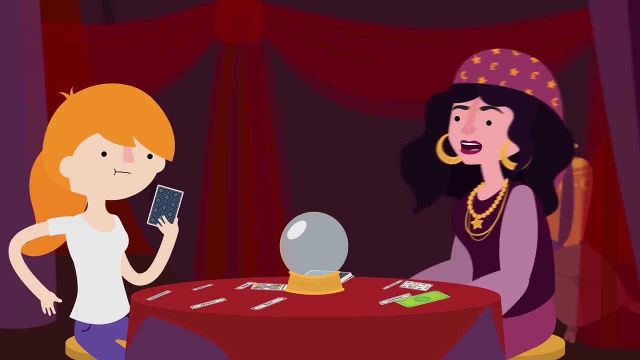 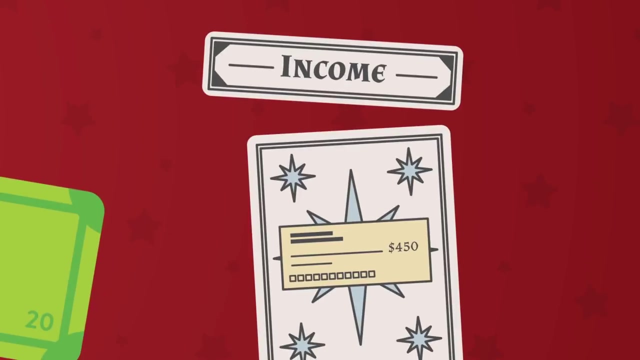 Oh no. What does it mean? Oh, that's just car insurance. That's usually an annual one, So that goes over here. Draw another. Oh my, With that card. I sense a powerful energy here. The utilities card. Wait, a second. Utilities income expenses. Are you budgeting me? 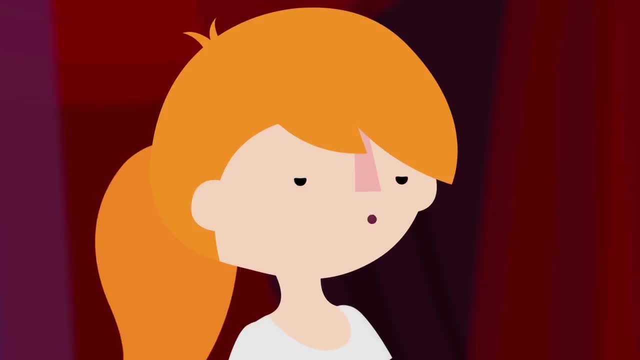 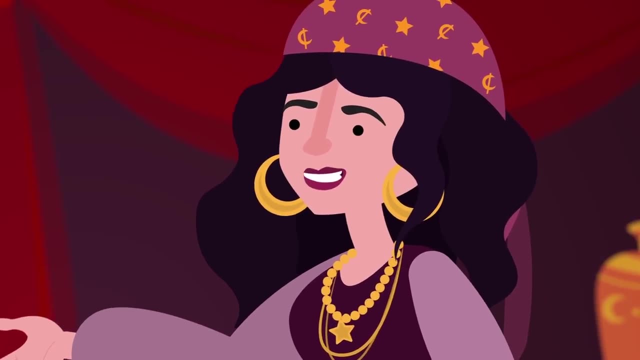 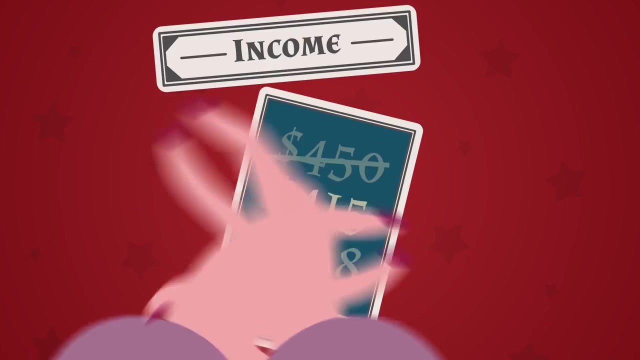 Well, yeah, I thought you read fortunes. You won't have any fortune left for me to read unless you know how much you spend versus how much you earn. Your income is actually less Then your paycheck or salary. When planning a budget, you must factor in taxes and deductions. 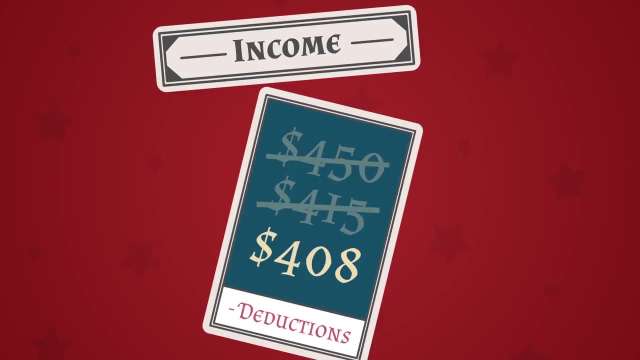 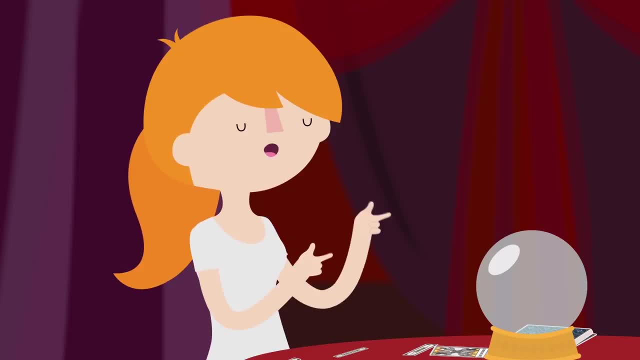 Otherwise you will be budgeting money you don't even have. But budgeting is mostly for saving up for big stuff. right, I pay my rent and internet and I still have money left over, So I'm good. How do you know what you can and can't afford? 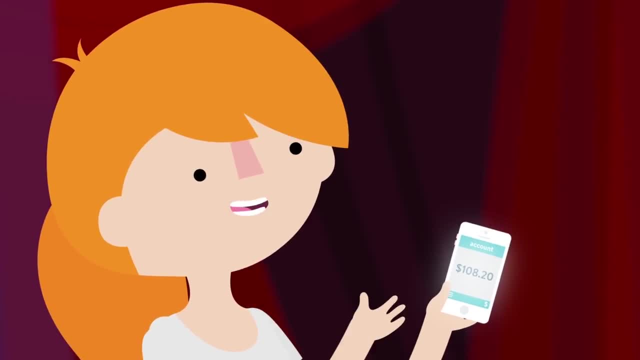 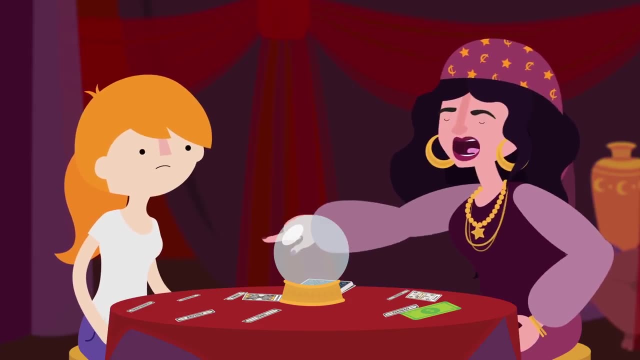 Um well, I look at my account balance and if there's money there, I know I can spend it. Your palm, Show me your palm, Palm reading. Now we're talking Ow: No more spending until you give every dollar. 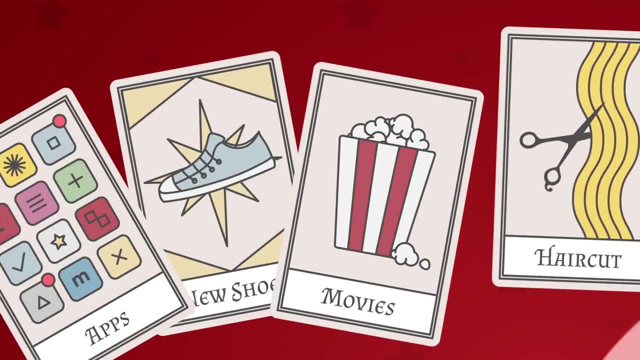 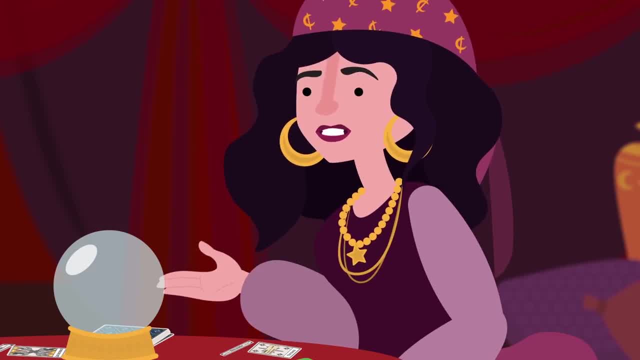 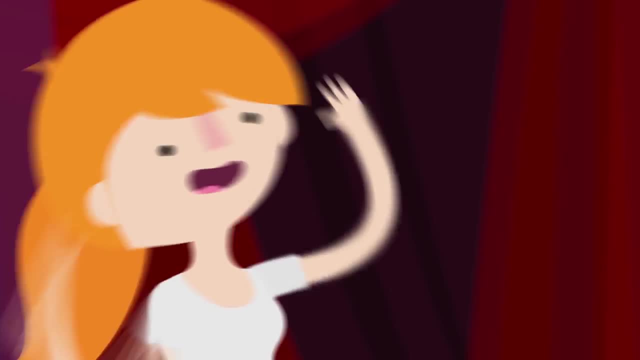 A job. Part of that account balance that you're freely spending on fun stuff should actually be going to savings and one-time payments. Budgeting doesn't mean feeling guilty for fun purchases. It means feeling confident about them, Like being in control of your own destiny.